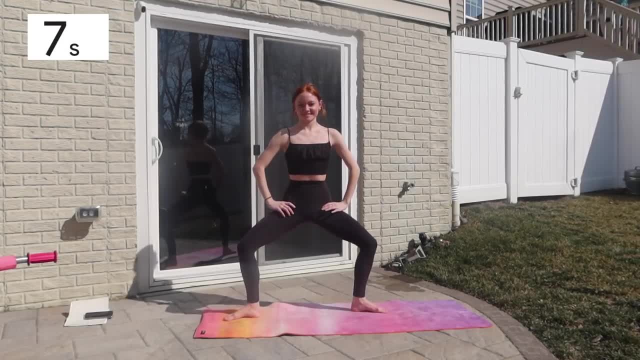 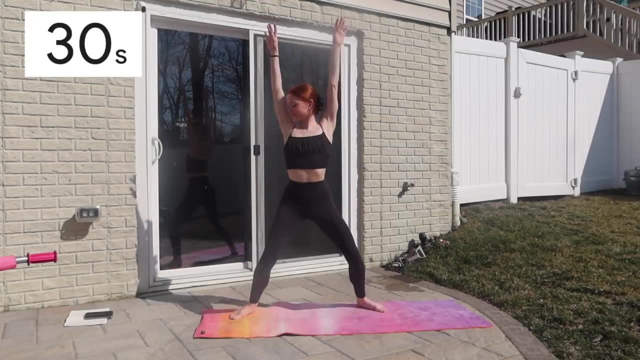 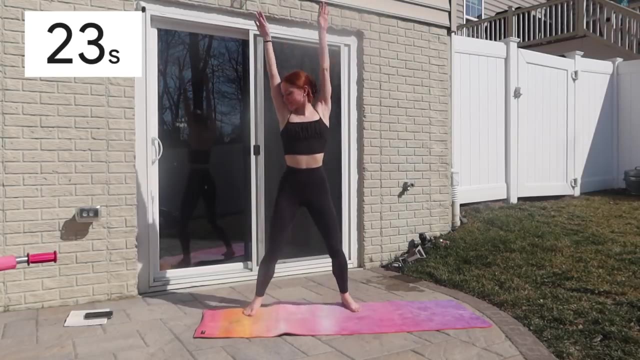 quad muscles. Soon, in the top left corner, you'll see a video of me of doing the next exercise, so you always know what's coming next. The next exercise is 30 seconds of jumping jacks, focusing on keeping our core tight and really jumping off the ground so we can get warmer faster. 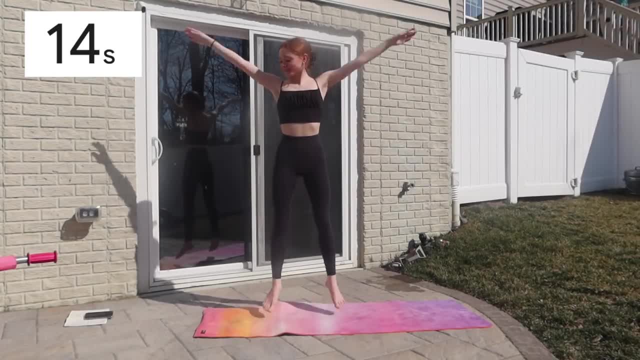 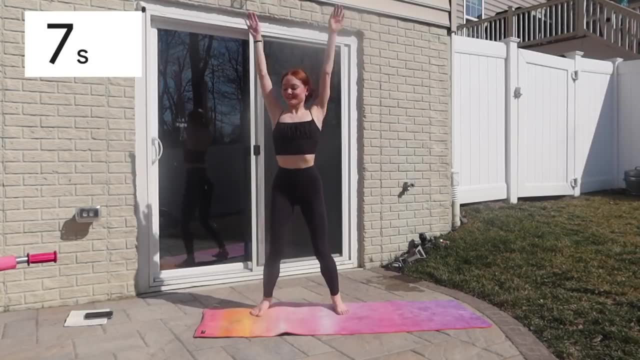 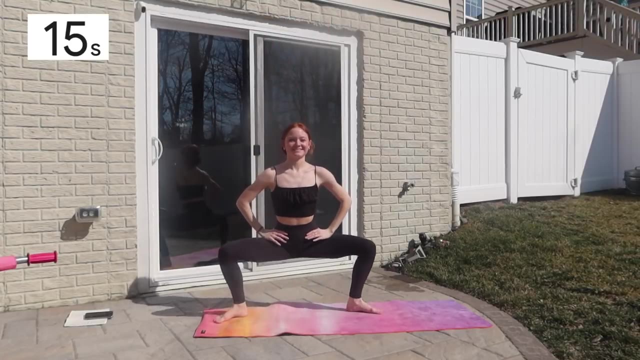 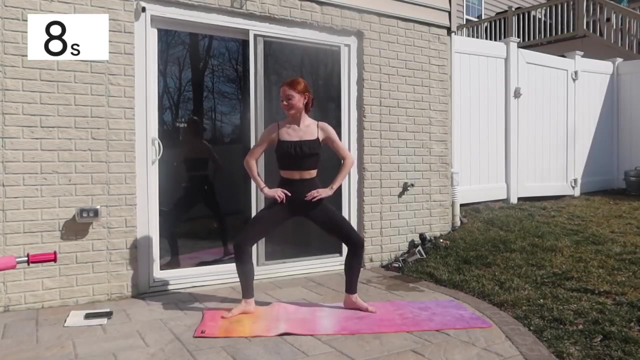 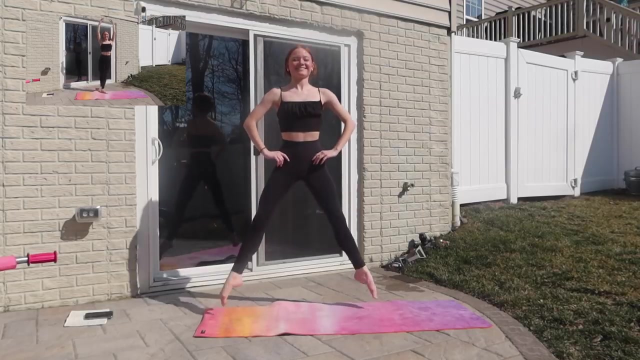 The next exercise are plie jumps. I know these look painful, but trust me, they get you really warm really fast. so just bear with me This next exercise. I'm not really sure what to call, but we're just going to switch our. 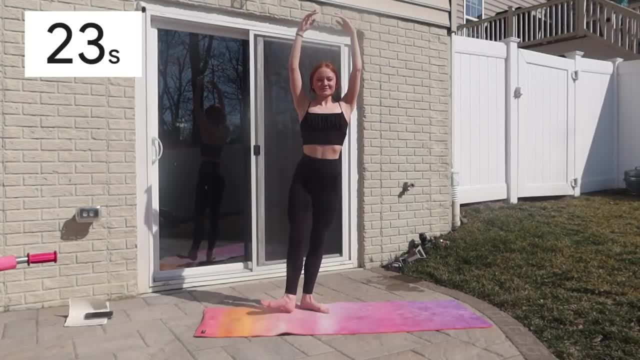 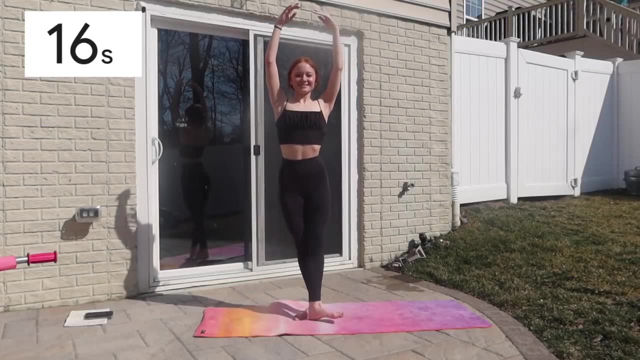 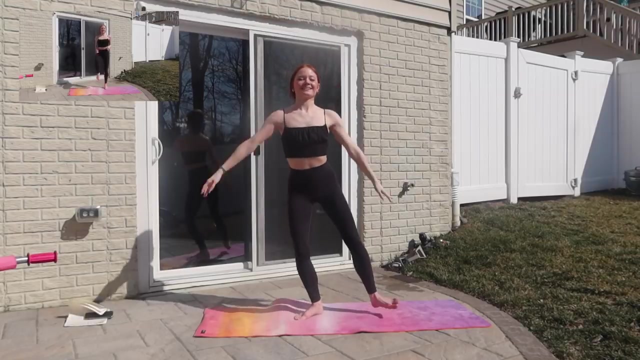 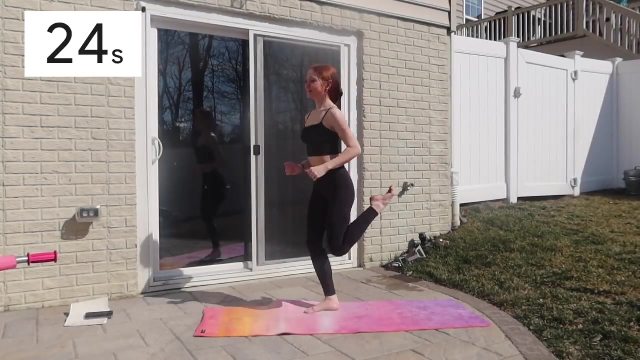 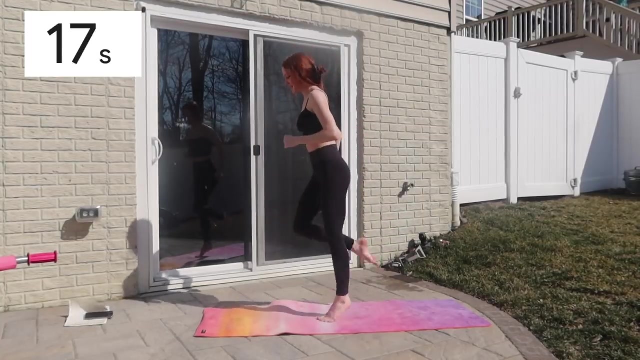 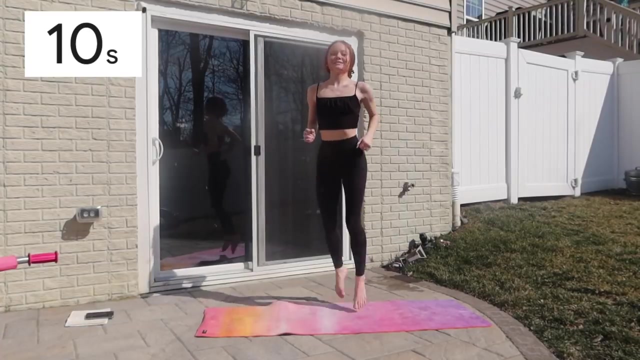 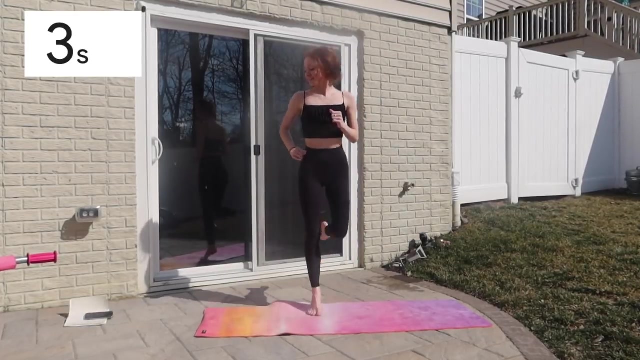 fifths while flexing our foot, and we're going to be switching our legs halfway through And switch to the other side, And our last exercise for the warm-up is just 30 seconds of running in place. Great job, guys. Now let's move on to stretching. 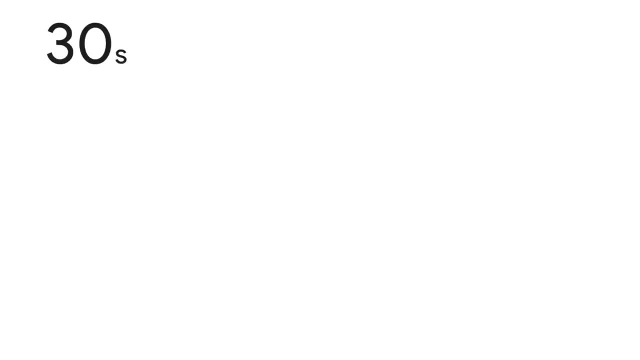 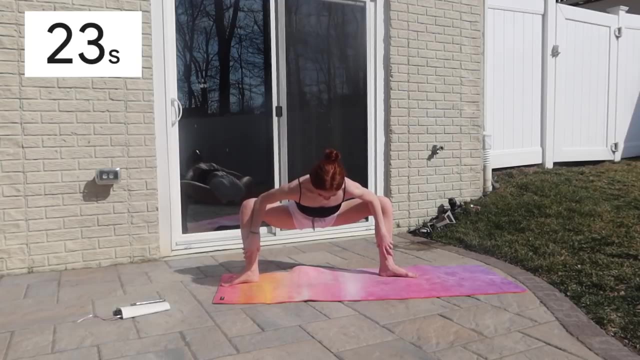 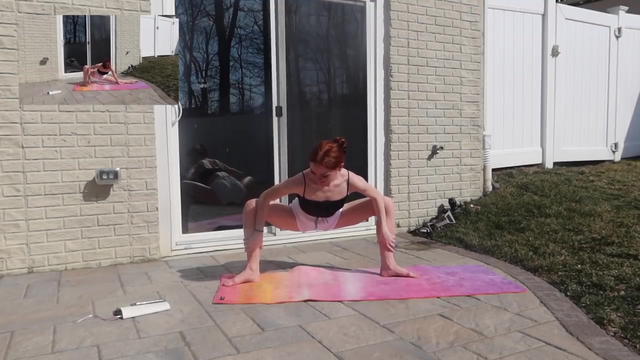 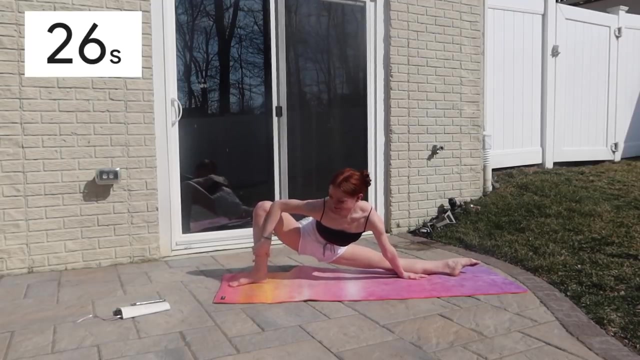 Okay, let's start stretching. So we're going to go down into a deep second position: plie and push our knees back with our elbows, Straighten that left leg and continue to push back your right knee with your elbow, and we're going to hold this for 30 seconds. 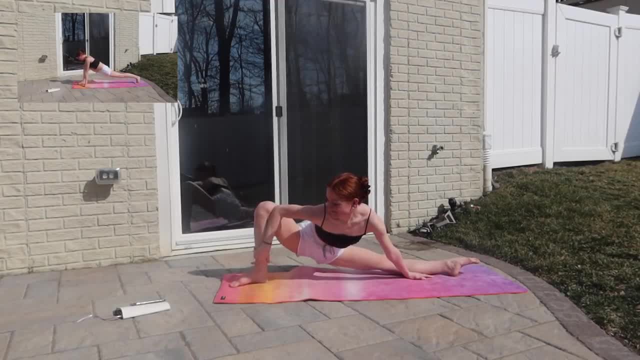 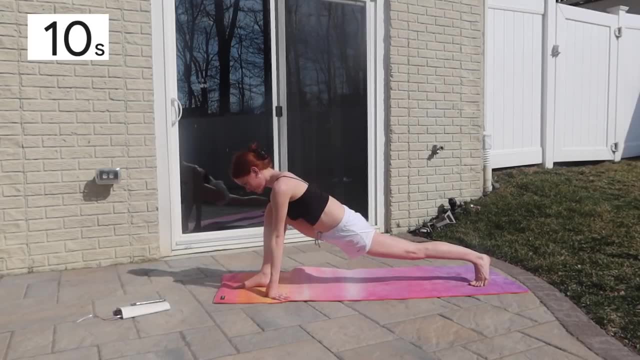 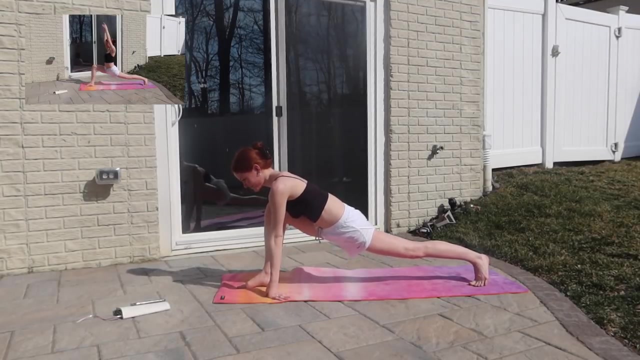 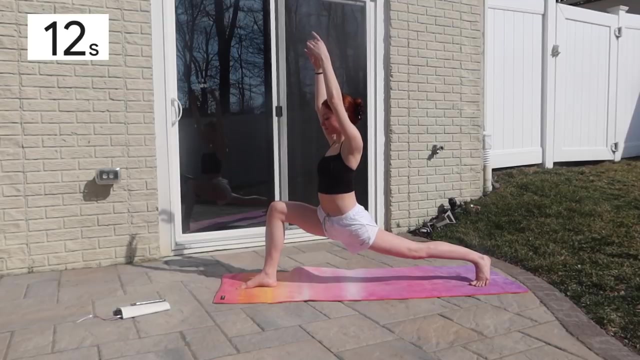 Now flip over to your lunge and really relax the hip flexor and we're going to hold this for 15 seconds. Now release those arms and put them above your head and continuing to breathe through that stretch and really releasing that hip flexor. 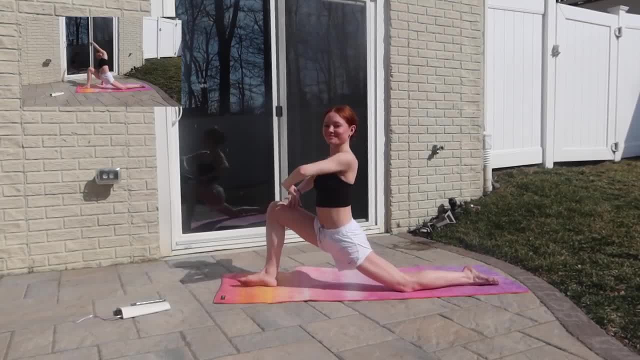 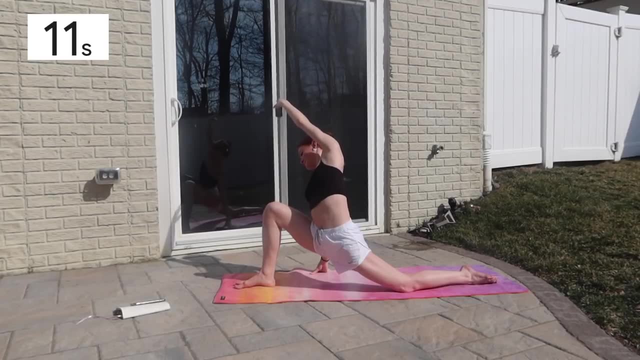 Now release that knee to the ground and take a big side stretch to the right. Okay, now come up and stretch backwards however you like, and please don't forget to release that hip flexor. it's so important. Okay, now come up and stretch backwards however you like, and please don't forget to release that hip flexor. it's so important. 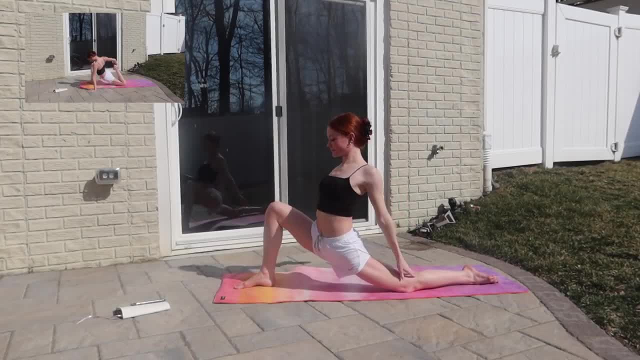 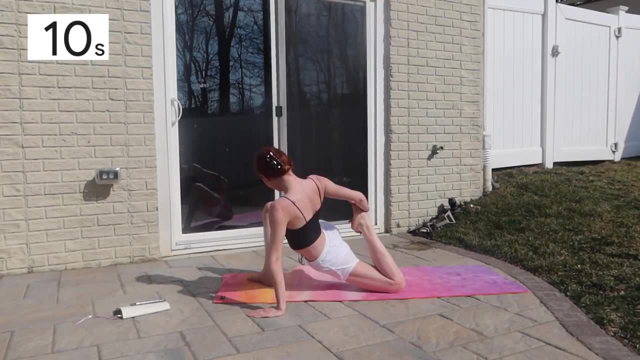 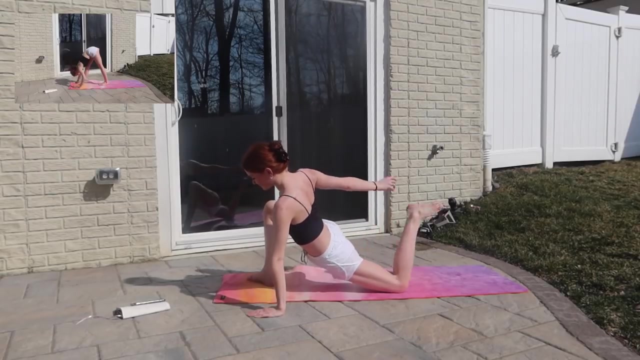 Okay, now come up and stretch backwards however you like, and please don't forget to release that hip flexor. it's so important. Okay, now reach back and pull your left foot into your tailbone. Okay, now reach back and pull your left foot into your tailbone. 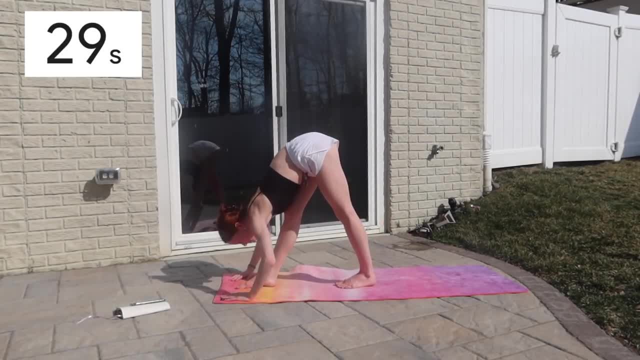 Okay, now we're going to scoot up into a parallel fourth position, and this is my personal favorite stretch, so good for the hamstrings. We're going to stay here for 30 seconds, Just remembering to release our hamstrings. Just remembering to release our hamstrings. 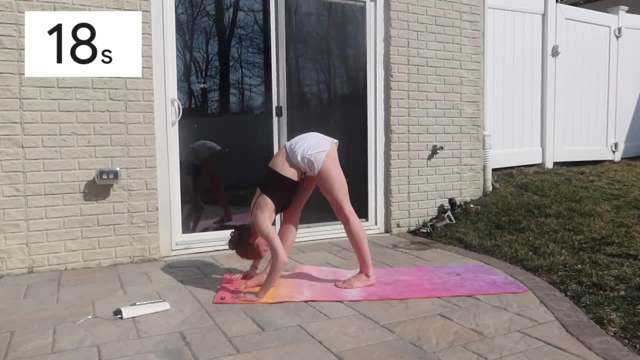 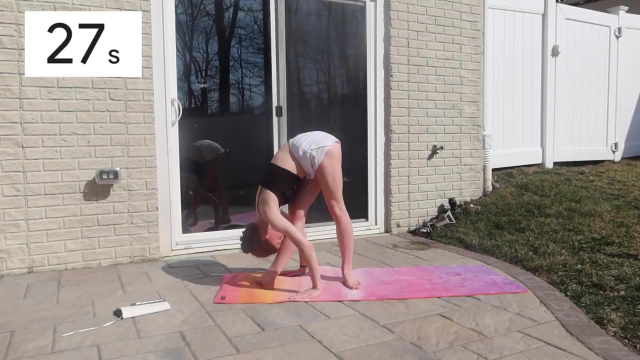 Just remembering to release our hamstrings And really get the most of this stretch. Now we're just going to turn out both of our feet and do the same exact stretch for 30 seconds. Now we're just going to turn out both of our feet and do the same exact stretch for 30 seconds. 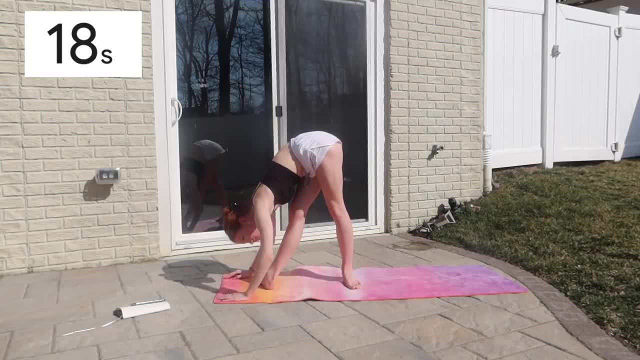 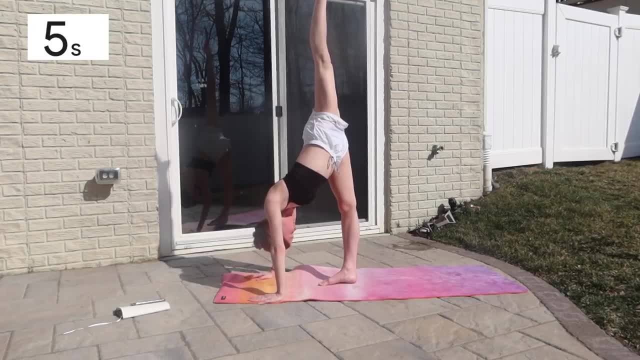 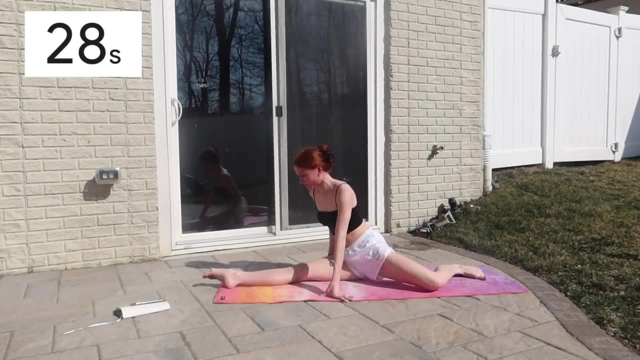 Now we're going to develop our left leg to the sky and really stretch our penche here. Now we're going to develop our left leg to the sky and really stretch our penche here. And for our last stretch, just go down into your right, split and stretch however way you. 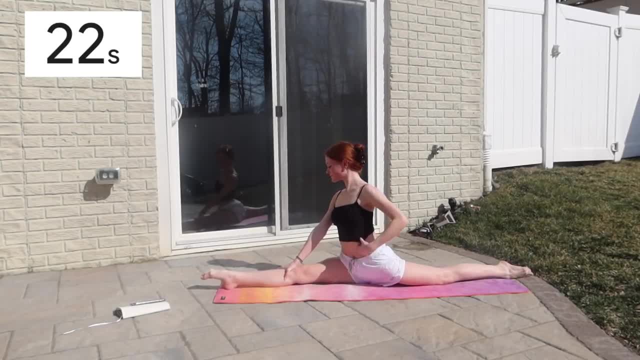 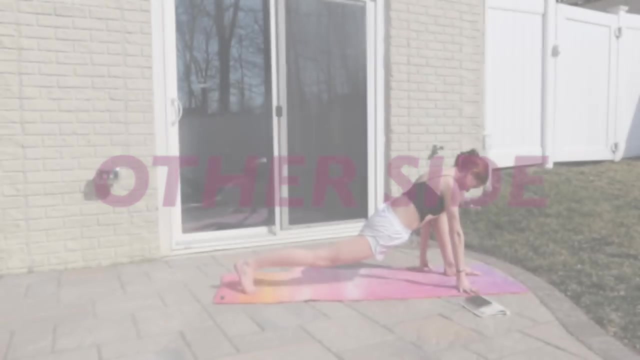 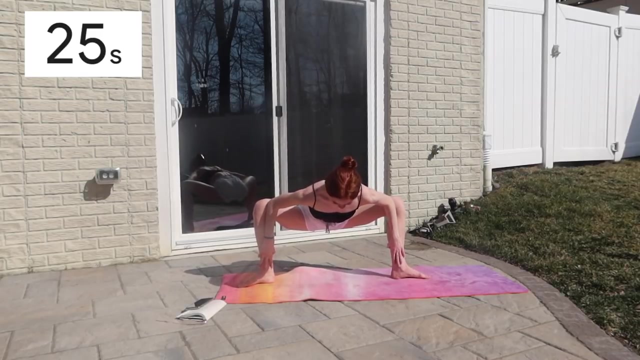 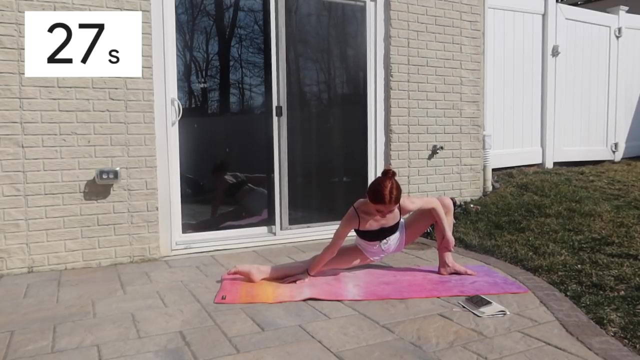 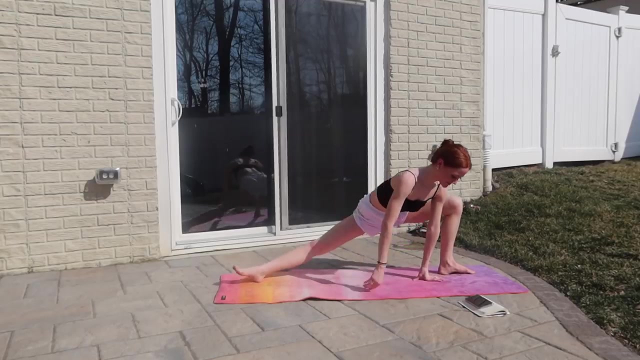 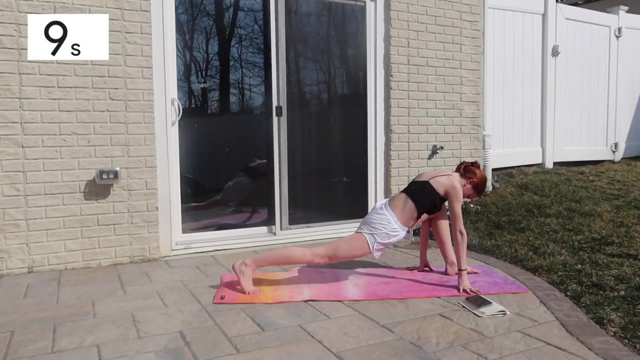 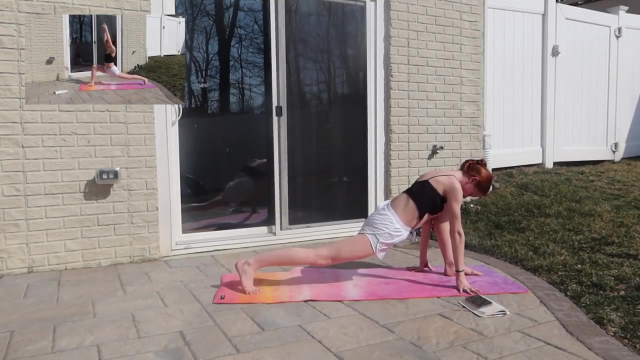 like in your split. Great job, you guys. Now let's move on into the other side, Going down into our deep plie. second position: stretch. Great job. Straighten the right leg and continue to press the left knee back. Now flip over to your left lunge. 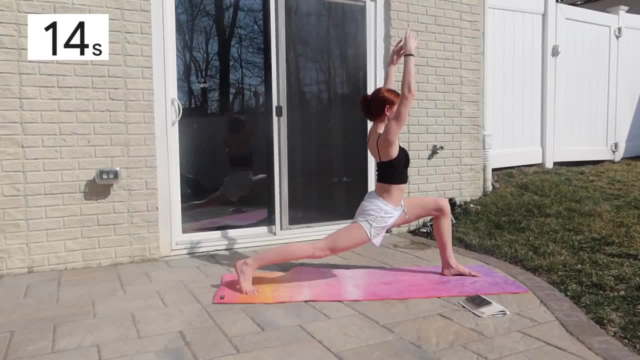 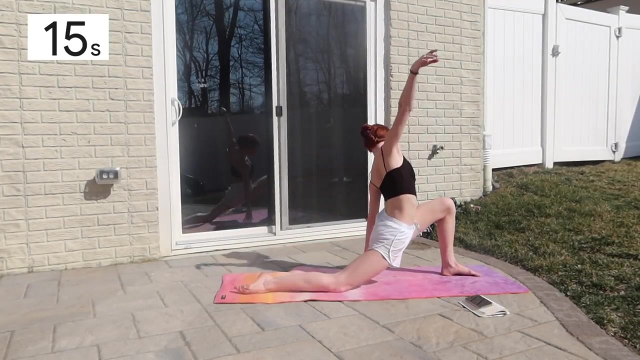 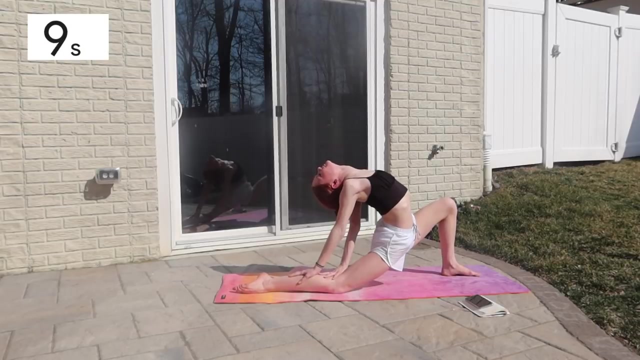 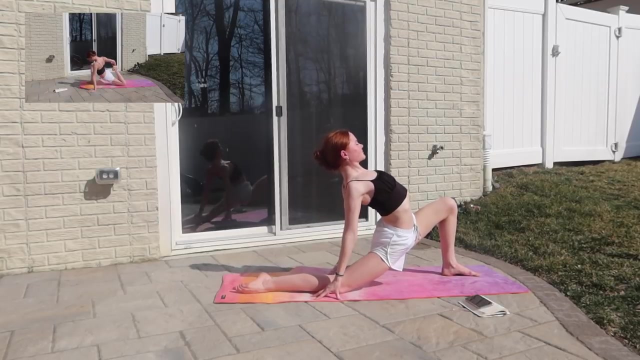 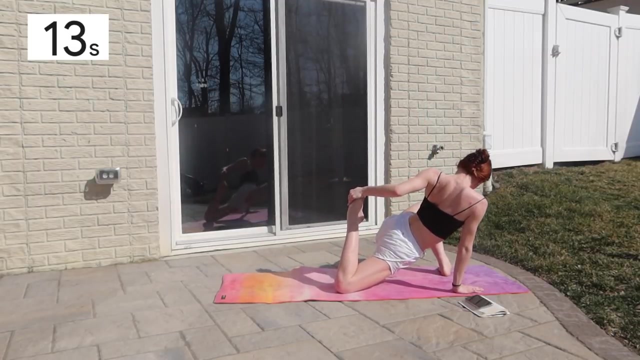 Press those arms and put them above your head, Release your knee to the ground and stretch over to the side. Now let's do the other side: Keeping that knee on the ground, stretch back to grab your leg. Now, reach back and pull that right foot in.